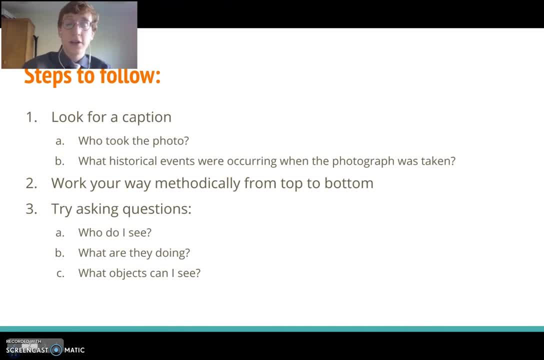 And sometimes they'll also have the date or who is included in the photo, And so from that you can determine what historical events were occurring when the photograph was taken and just get better context to use when analyzing the photo. And you're going to want to work your way methodically from top to bottom when analyzing a photo. 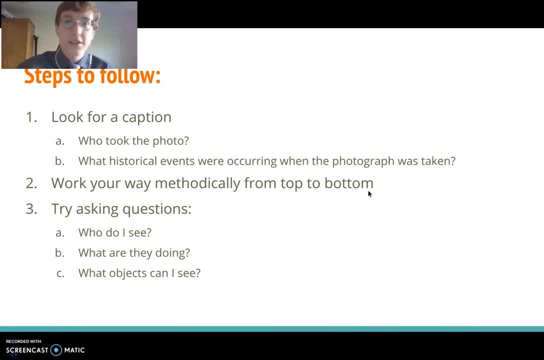 A lot of times it can be really tempting to just look at the first thing you see on the photo. That can cause you to focus too much on one thing and miss important details in the background. So you want to go top to bottom, left to right, just to make sure you don't miss anything. 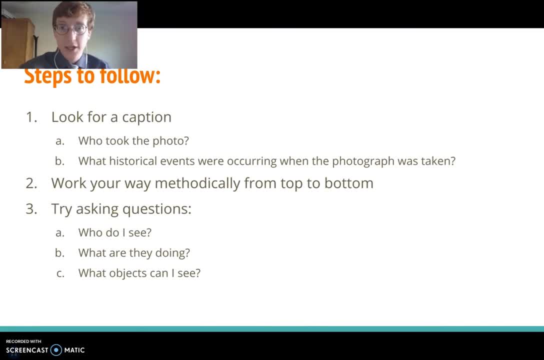 And as you're doing that, you should keep three questions in mind: Who do I see, What are they doing And what objects can I see? And this is just going to help you decode the important things from the photo and determine what the photographer is trying to convey by taking them. 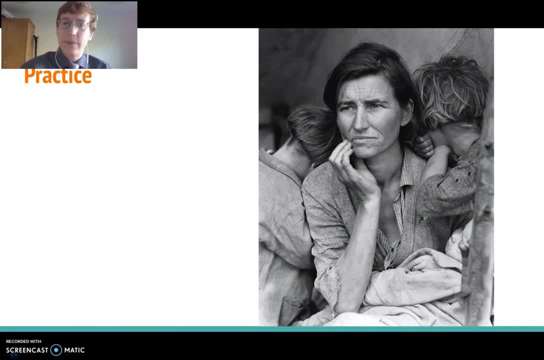 So now we can do some practice here. This is a pretty famous photo some of you might be familiar with. It was taken by Dorothea Lange and it did come with a really great caption She said: Destitute pea pickers in California, mother of seven children, age 32, Nipomo, California, February 1936. 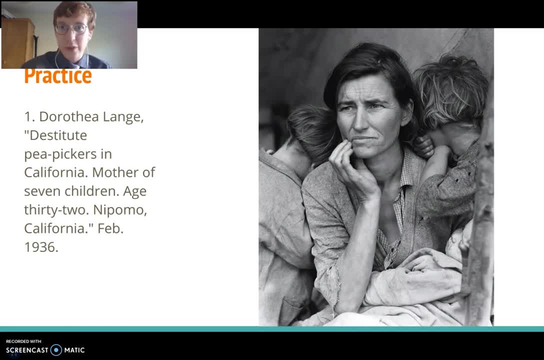 So already, even before looking at the photo, just because we took the time to read the caption, we know loads of information. So we know where they are: they're in California, we know who's in the picture and we know when the picture was taken- 1936. 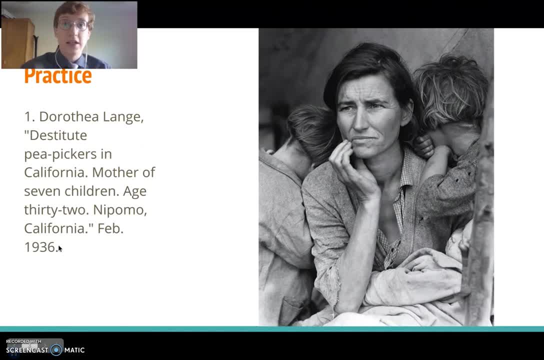 And so from that we can do a little historical inferencing. This is taken during the Great Depression and they're destitute, so probably these individuals were affected by the Great Depression. So remember, when we're looking at these photos we want to go left to right, top to bottom. 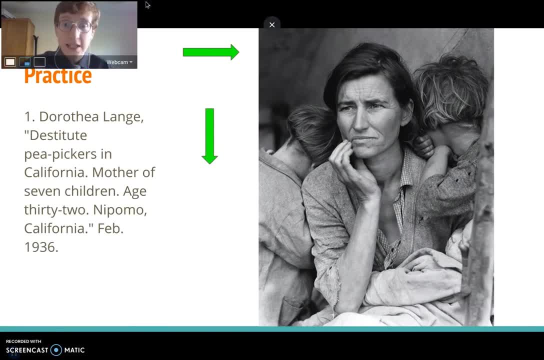 just to make sure we don't miss anything. So as I'm going through this, there's not a whole lot in the background. there aren't really any objects I can see, so that question's kind of out, But the first thing we see- who's in the photo? 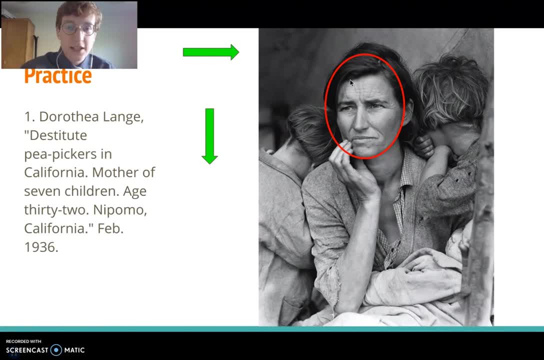 we see the woman. the mother is prominently displayed and we know she's 32 from the description, but she's looking pretty wrinkled, pretty concerned, maybe like she's aging more rapidly than is normal. So that's kind of hinting at the fact that her living conditions aren't great. 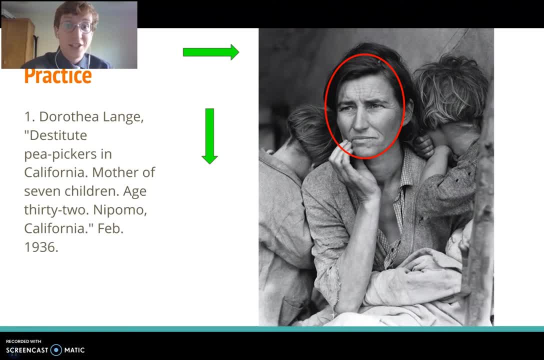 her life's maybe not the best. she's obviously worried about things. she doesn't look happy, so that's important to know. Then we're scanning left to right, going down. Next thing we see is this child's hand. It's looking pretty dirty, which isn't totally unusual for children. 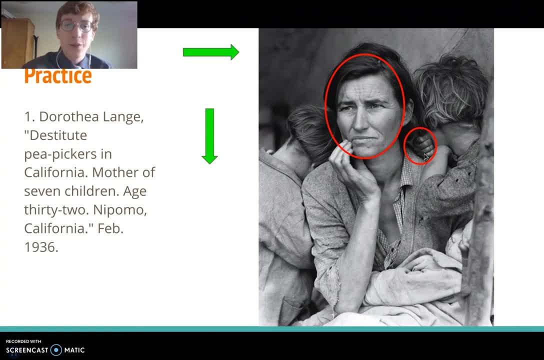 but again this could be a sign of poor hygiene or lack of hygiene. but again this could be a sign of poor hygiene or lack of hygiene or lack of access to hygiene facilities. Maybe he can't wash his hands and that's contributing to what Dorothy said in her caption. 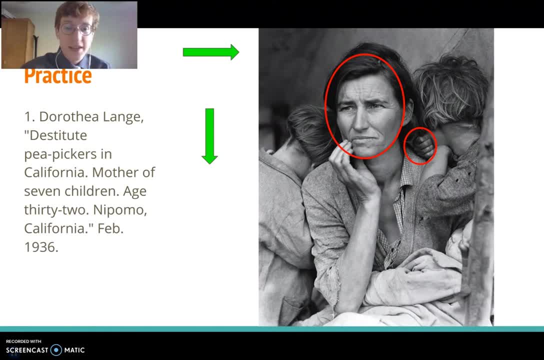 which is they're destitute. these people are impoverished. As we keep looking, we can find further evidence of this. He has holes in his clothing here and here, so now we know they don't have enough money to even buy new clothes. 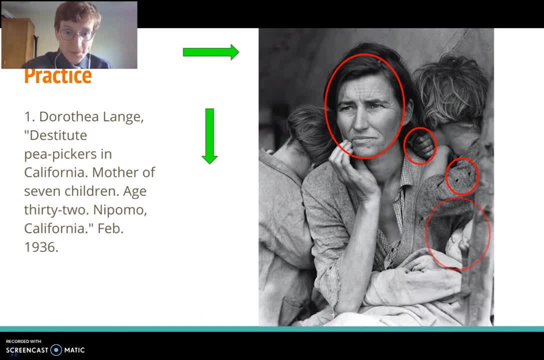 So that's good. As we keep looking, there's actually a baby. She's holding a baby. This is the first time I went through the photograph And if you look really closely at the baby you can see they have dirt on their nose and on their face. 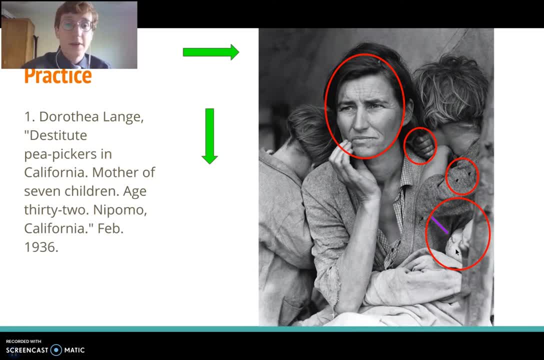 again contributing to the notion that these people maybe don't have access to proper facilities. they're living impoverished, really not a great life. So we know they're affected by the Great Depression and these are the signs of it, And then, finally, there's just some tattered clothing. 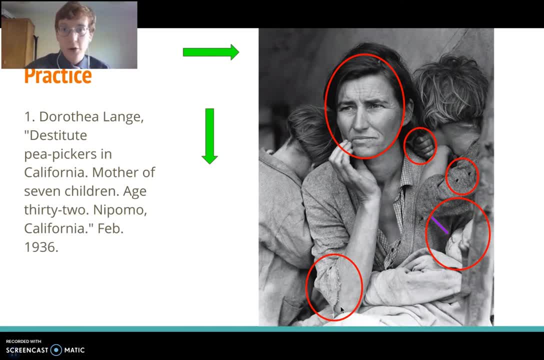 So in doing that, we answered our three questions. Who's in the photo? Our mother and the baby, and then also the two boys in the background. We can't see too much about them. Objects: There aren't many objects besides the clothing. 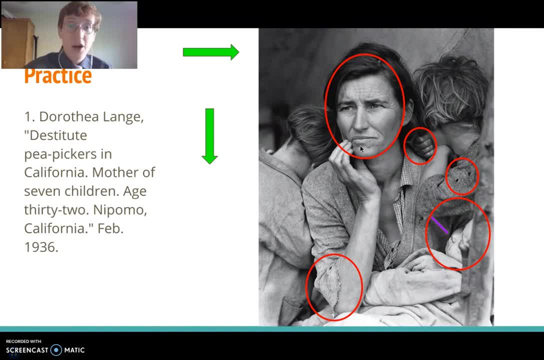 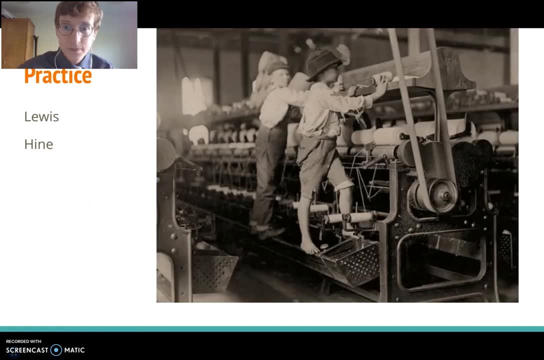 and then they're not really doing anything, so we can't answer that question. But again, we've already learned a bunch of information just from going through methodically and answering our three questions, So let's try this again. So this is another photo taken by Lewis Hine. 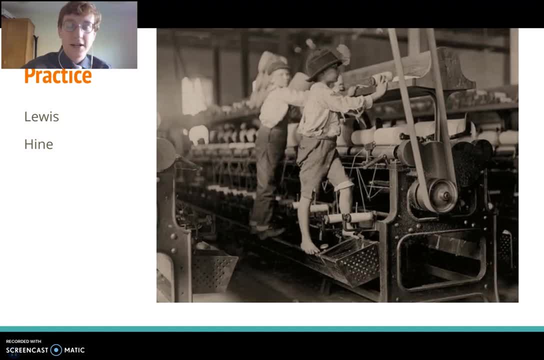 He's not quite as famous around in America, but still super important. So, looking at this photo, we're going to do the same thing we did before: Left to right, top to bottom. So we're scanning. The first thing I noticed was this conveyor belt that starts in the top and goes on down. 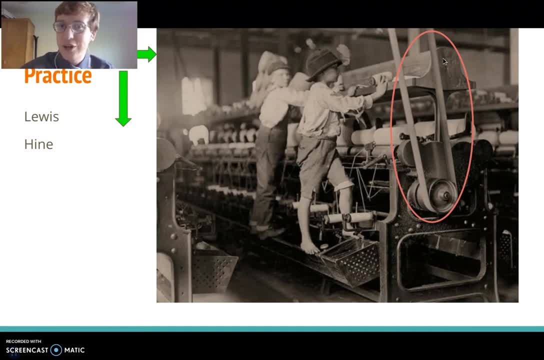 It's exposed, it's looking pretty dangerous. so that's kind of giving us a hint that, hmm, maybe this photo wasn't taken very recently because hopefully there'd be better laws about having dangerous things like that exposed. Then, as we continue scanning, I notice that there's really only one window that we can see. 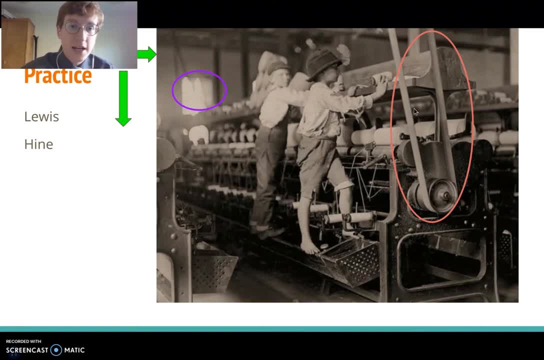 and I mean obviously it's blocked partially by the machinery, but this is kind of giving us the idea that maybe they're in a factory or some kind of manufacturing plant. Then we look over at our two boys. I just highlighted him because he's a little easier to see. 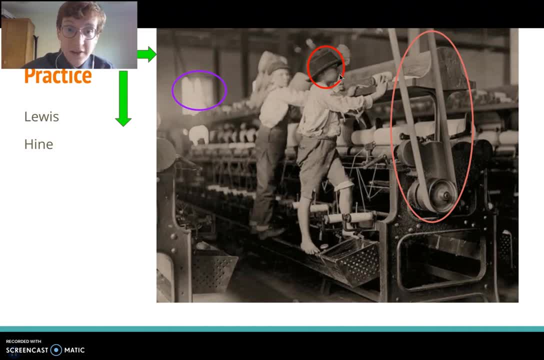 And they're looking very young. We can tell by their face They can't be very old. So that's again contributing to the fact that this photo is probably pretty old, because obviously this is child labor. so we know that this took place in the middle of the year. 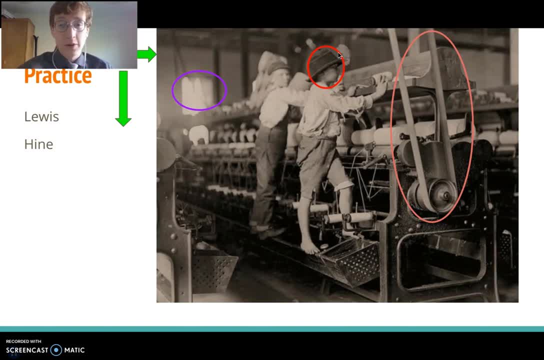 we know that this took place before child labor laws were put into place and most likely, you know, when we put that together with the conveyor belt, this was probably taken during the Industrial Revolution. And again, there's just some more bobbins in the back. 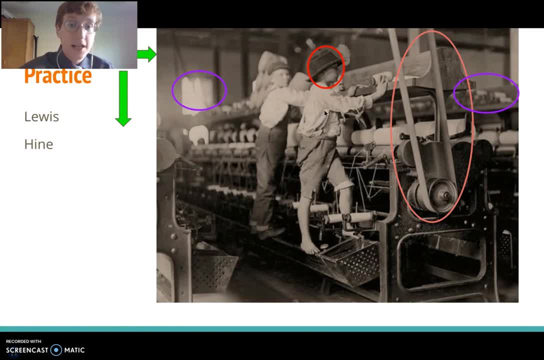 and you can see lots of machines. Again, probably during the Industrial Revolution things were being manufactured, So that's great. We already have a bunch of information from that, but we're going to continue scanning. and we notice he's got tattered clothing here. 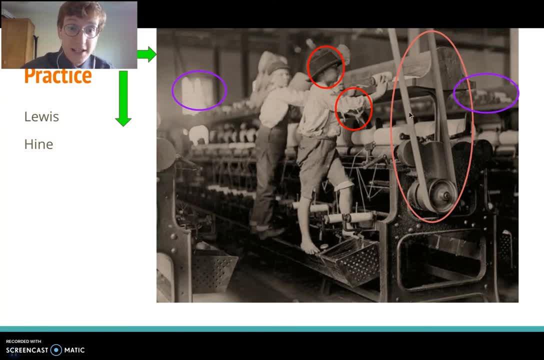 which is probably pretty dangerous, considering he's right next to a belt that that could be caught up into. You know, he's got a rip in his jeans and he's barefoot, So we can probably assume that the child in the front is again impoverished. 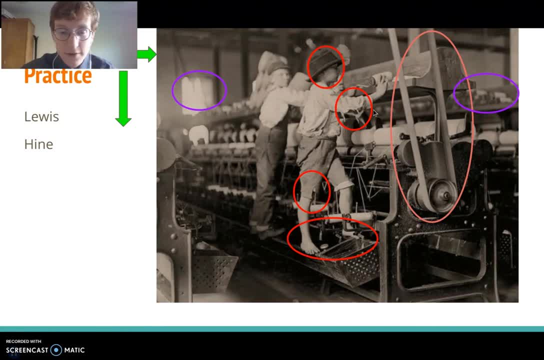 He doesn't have a lot of money. he can't buy himself new clothes, can't even afford himself shoes. The other thing we notice, though, is he's standing on this basket here just to reach this upper shelf, indicating that he's small enough that he can't even operate the machines correctly. 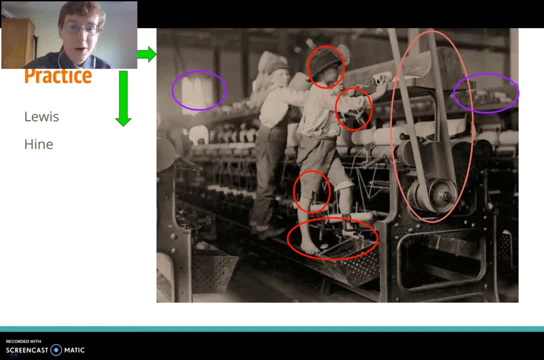 indicating that he probably shouldn't be working. It is still a little bit of a risk for us as well. But again, this is just not the end of the conversation. We don't have much time, but it's probably best that we stick to the process of creating something. 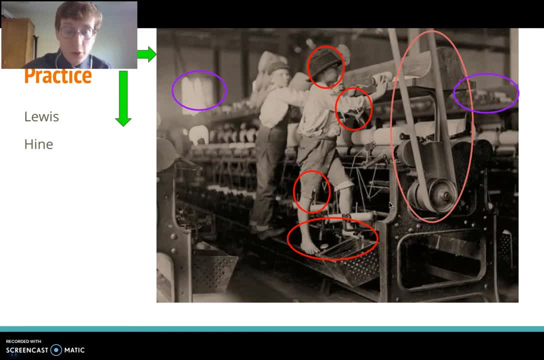 that he can finally take out and immediately use as his new home. So I'm just going to stop here and keep Quelan running. We'll be back in a minute with new statistics and new videos. All right, thanks, Bye.